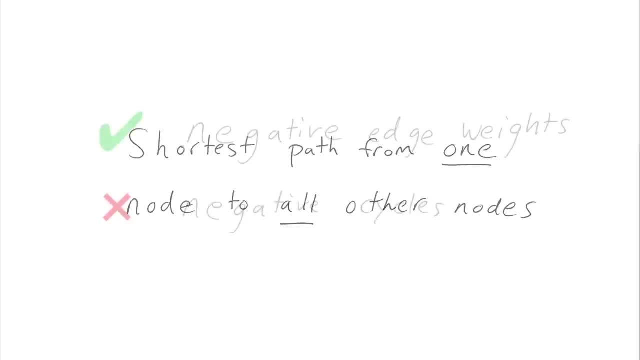 prims and Kruskals result in minimum spanning trees. The most important difference between the two algorithms is that Bellman-Ford works on graphs with negative edge weights, while Dijkstra's does not. However, both fail on graphs with negative cycles because in this case, a shortest path doesn't exist In a 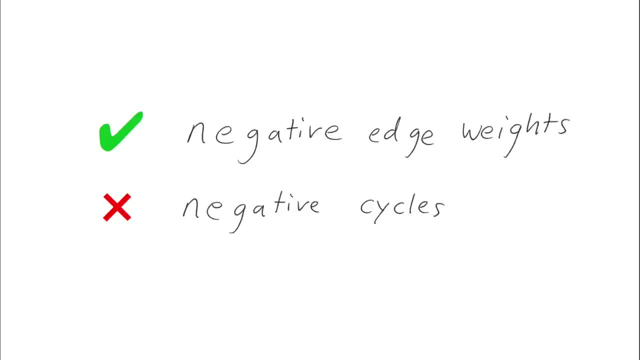 negative cycle. you keep going around the graph. In the second graph you kind of have a celui. So your average path in Dijkstra's is not marked with a sinonimate box. In this example, whose bets are second, Dijkstra's jacket is determined by the point of our 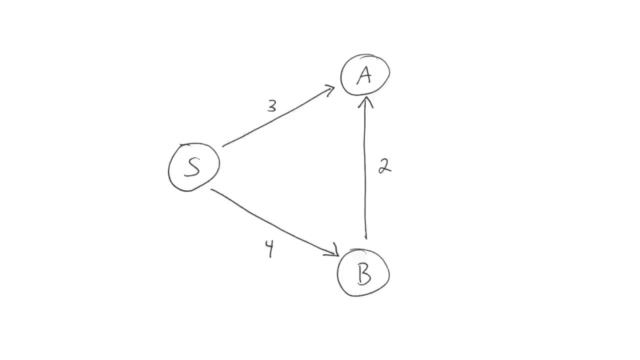 lessons, while Bellman-Ford's puppets are determined by numbers. That's what the first step here means. What did that fix? Nada, Old amias close it. so no more updates can be done on the path to A. But of course we know the. 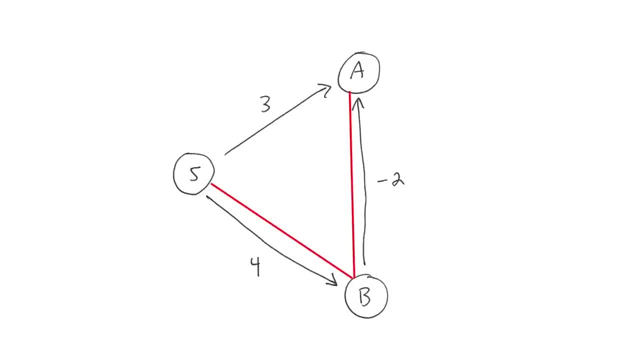 shortest path to A is now 2, and goes through B. This is where Bellman-Ford comes in. I'll use the following graph to explain the theory behind Bellman-Ford. Say, we want to know the shortest path from S to D. How would we do this? Well, we'd. 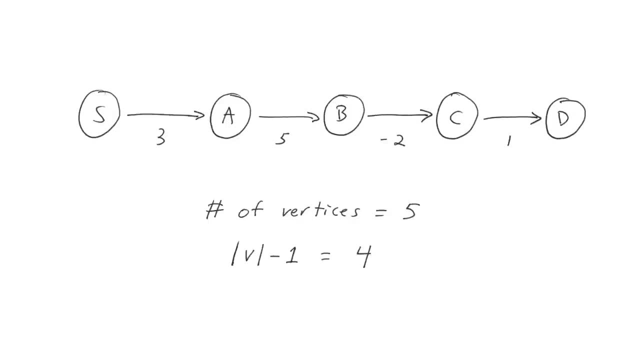 iterate 4 times, each time adding the edge weight to our path-length. Where did we get 4 and why is it important? This is the fundamental idea behind Bellman-Ford. There can be at most b-1 edges in a path from the starting node to any other node in the 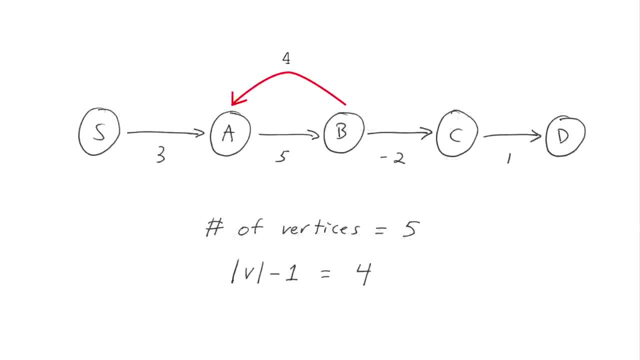 graph. Why is this? If someone told you the path from S to D had 5 or more edges, there would need to be a loop from one node to another node. so that's already in the path, aka a cycle. Since we know this can't be a negative cycle. 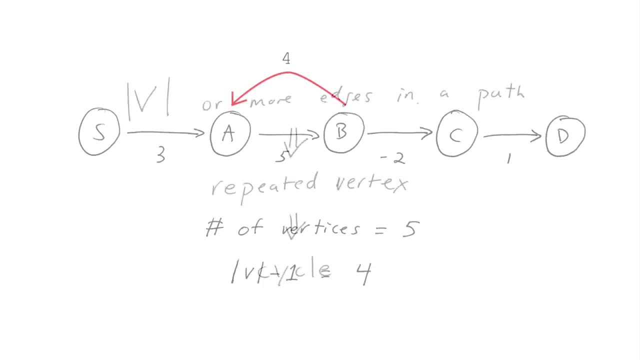 we could take out this edge to lessen our distance One more time. v or more edges in a path means there is a repeated vertex and therefore a cycle. All paths are said to be simple. Getting back to our example, we know if we iterate v minus one times, we're guaranteed to find the